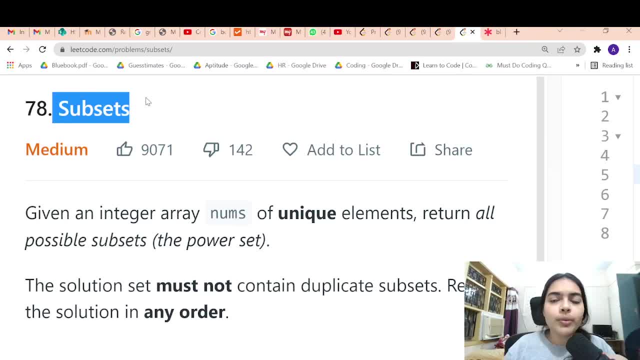 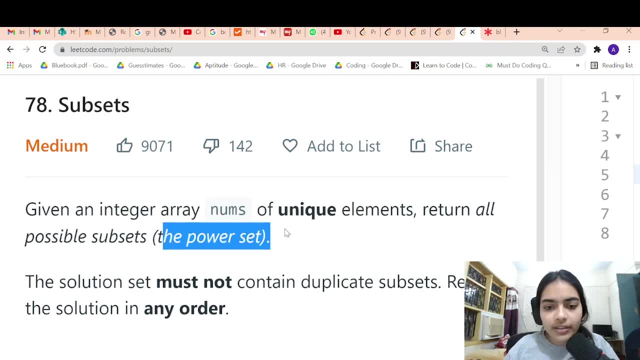 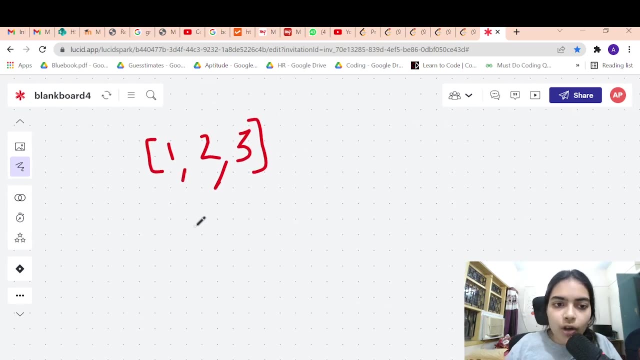 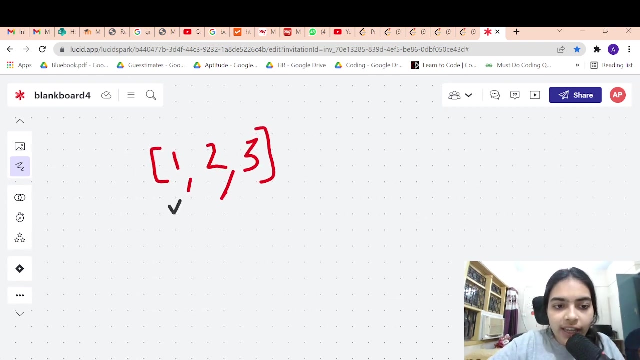 Hello guys, welcome to another video in the series of coding We are going to do the problem which is called subsets. So, given an integer array, nums of unique elements, you have to return all possible subsets, which is called the power set. Let's try to take an example to understand. Suppose you have 1,, 2, 3. If you want to generate all possible subsets of this, how will you generate? So, how to generate a subset? So, at every step you have two choices: You can take the first element or you can not take it. Similarly, for the second element, you have two choices: Either take it or not take it. 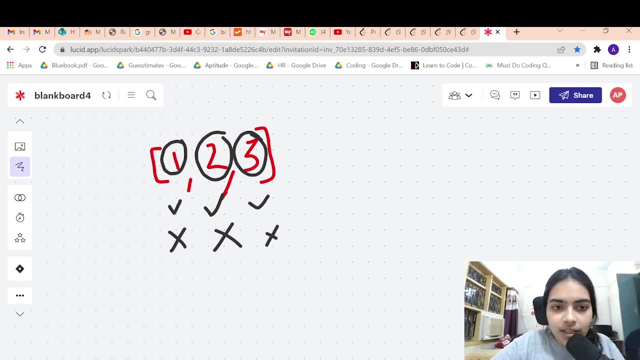 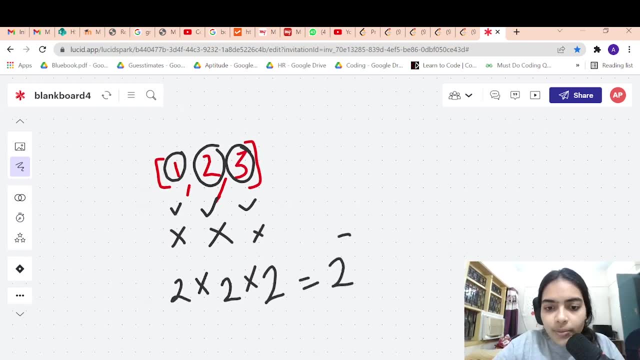 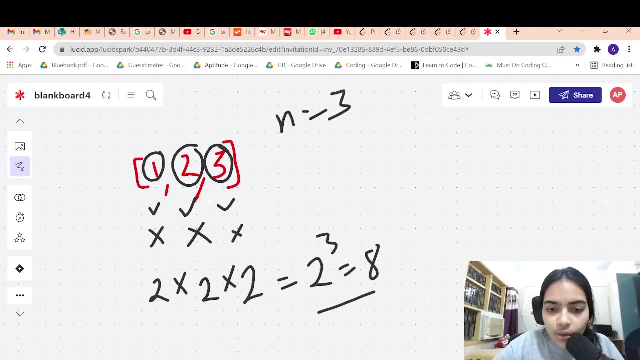 For the third element, you have two choices: Either take it or not take it in the subset. So you have two choices for the first element, two choices for the second element, two choices for the third element. So how many subsets will be there? Totally, you will have 2 power 3, which is 8.. Here n is equal to 3 because there are three elements. So for n equal to 3, you have 2 power 3 subsets. For any n, you have 2 power n total subsets, Because you always have two choices: Either take it or not take it. What do we mean by that? 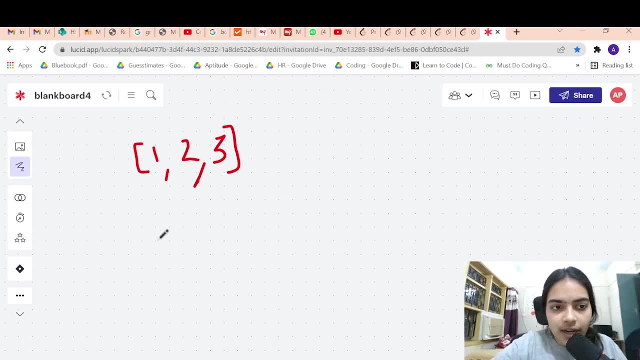 See, it's very simple. Let's try to generate all possible subsets. Let's say we take the choice We are not going to take any of the elements. This is one possible choice that we can make. So in this case you will generate an empty subset. If I don't take any of the elements, I will generate an empty subset. Let me take the next choice. Let's say I take only the first element and I don't take the next two elements, So I will get the subset 1.. 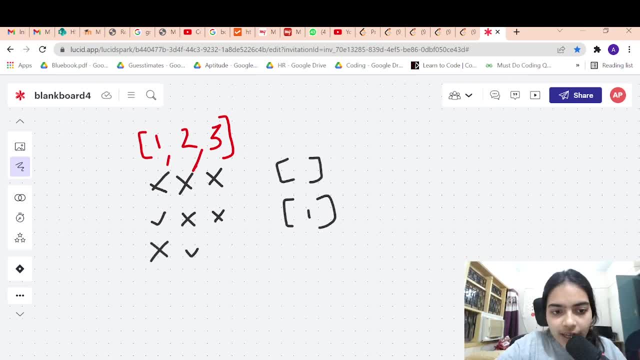 Next choice that I have. let's say, I don't take the first element, I take the second element. I don't take the third element, I will generate the subset 2.. Similarly, if I don't take the first two elements, I take the third element. I will generate the subset 3.. 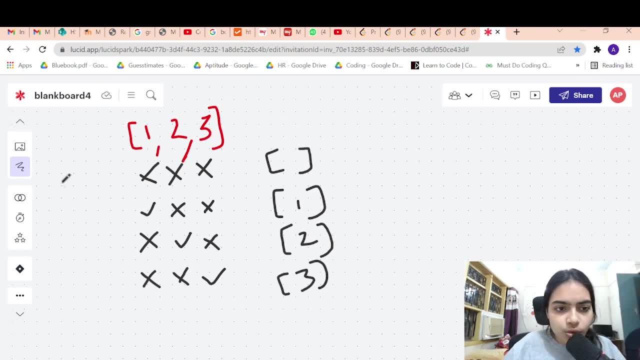 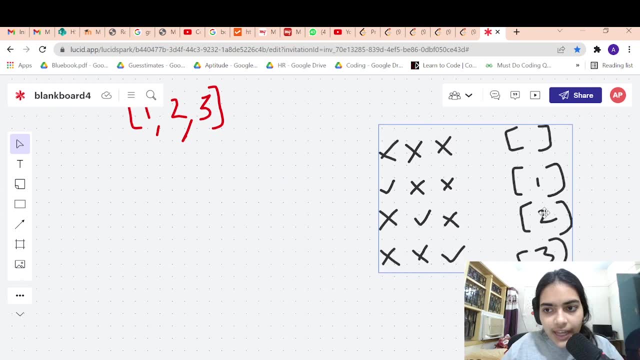 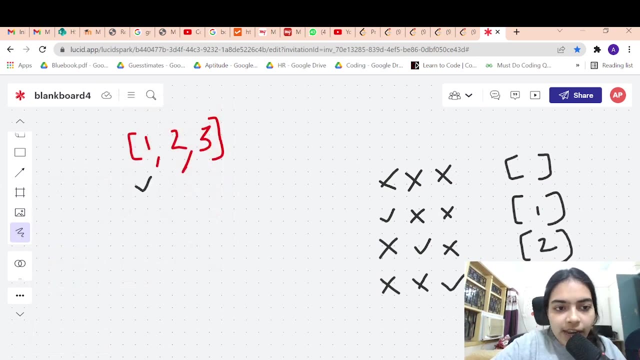 Next choice, what I can have. let's say I decide to, so let me do one thing, Let me just shift these on this side and let's write the next possible choices that we have. So now let's say we decide to take two elements and we don't take the third element, So the subset we generate is 1, 2.. 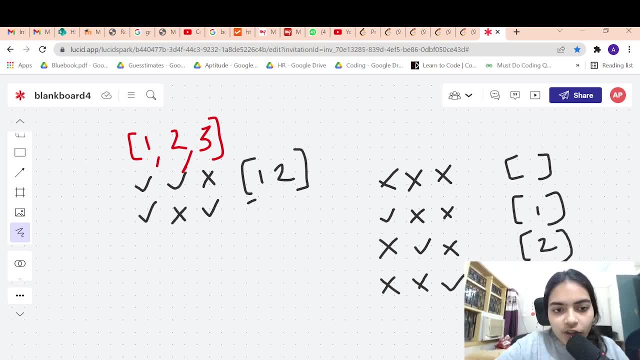 Similarly, let's say we decide to take the first and the third element and we don't take the second element, So we generate 1, 3.. Let's say we decide to take 2 and 3 and we don't take the first element, So we generate the subset 2, 3.. 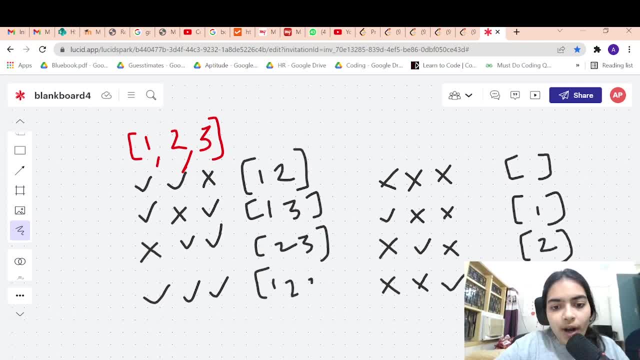 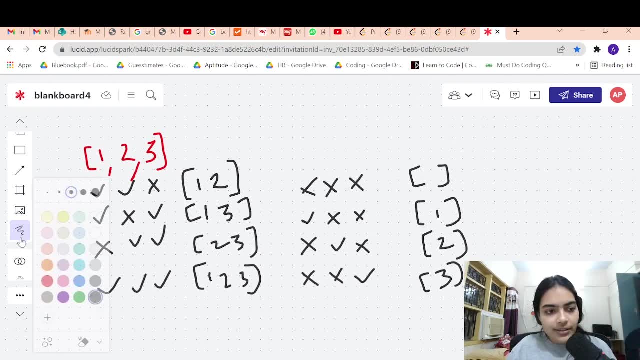 Now let's say we decide to take all the elements, So we will generate the subset 1,, 2, 3.. So these are all the possible subsets through all the possible combinations. So what we were doing is very simple. 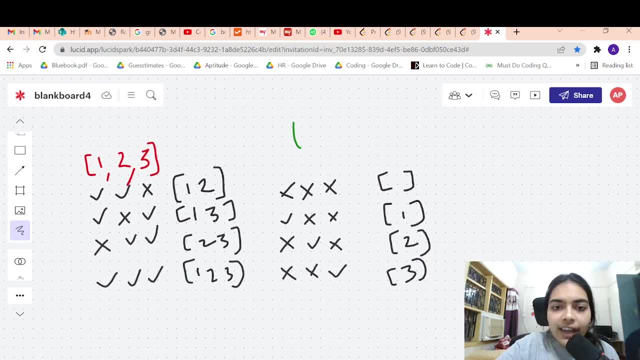 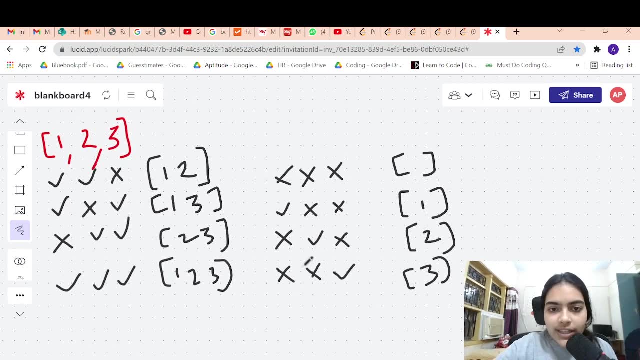 So we have a choice that we have to make at each step: Either take that element or don't take that element. So see, if we just use a binary representation instead of choices, right, if we just use a binary representation, for example, this just means 0, 0, 0. 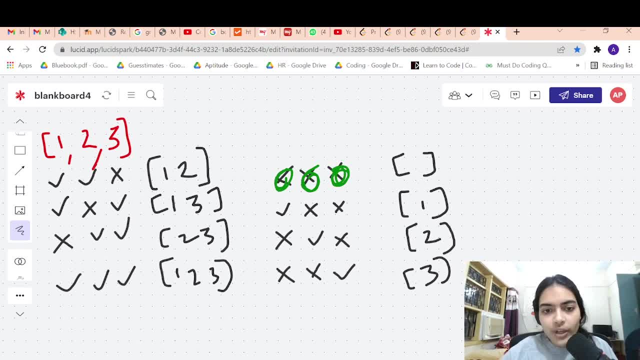 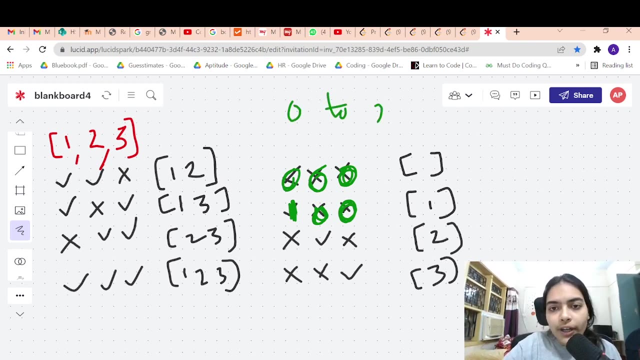 Whenever we are not taking element. this is a binary representation of 0, okay. Similarly, if, instead of you know, taking the element, I write 1 and not taking the element, I write 0, right. So this is again a binary representation. So I can use binary numbers from. I can use binary numbers from 0, okay. to 2. power n. 2 power n not included: right. 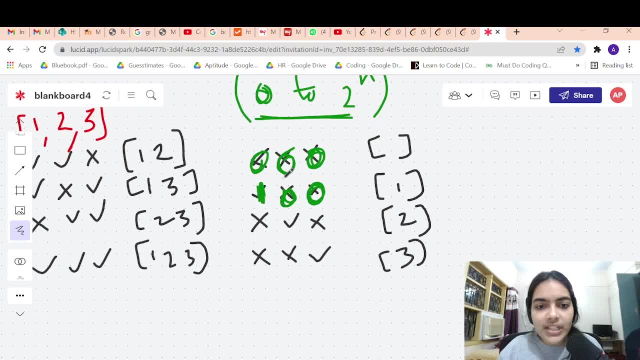 So between 0 to 2 power n. if I take 2 power n binary numbers right, I will be able to get all the subsets. okay, Let me write it, then it will be much more clearer. See, this is the representation for 0.. 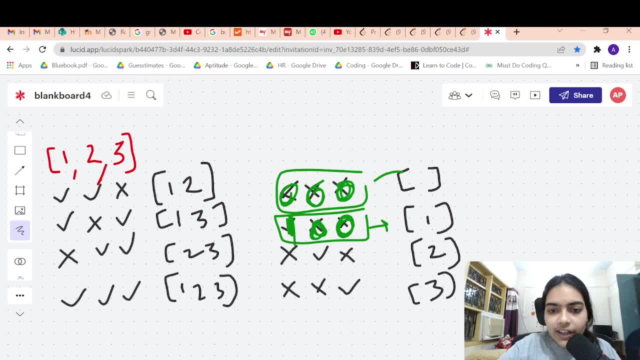 If I take 1, 0, 0, means I am taking the first element, not taking the next two elements. I get the subset 1, okay. Similarly, if I write 0, 1, 0,, this is also a binary representation of one of the numbers between 0 to 2. power n right. 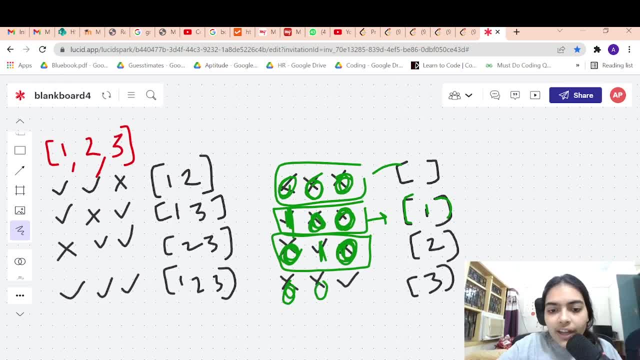 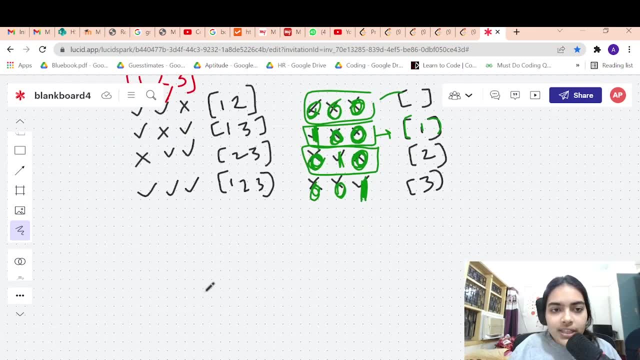 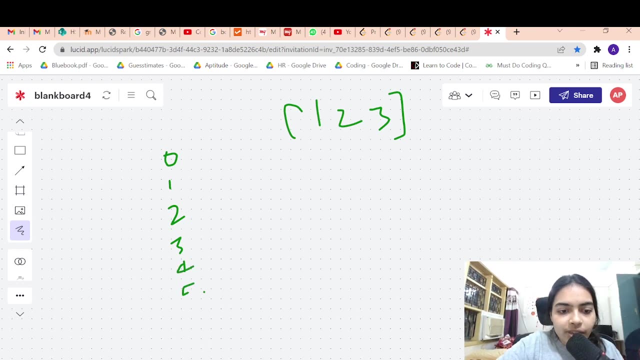 So if I write, I get this. Similarly, if I write the binary representation of all possible numbers- right, I just convert these to binary representation- I will be able to form the subsets. okay, See, let's try to write it properly. See, I write all the numbers from 0, okay, I write all the numbers from 0 to less than 2. power n- right. 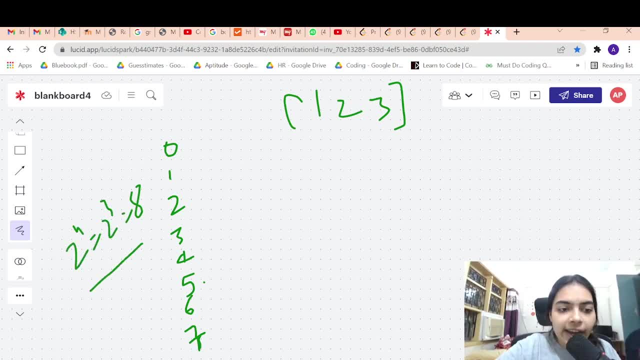 2 power n is equal to 2 power 3, which is equal to 8.. So I write 8 numbers, from 0 to 7, okay, And I write the binary representation. What is the binary representation of 0?? It is simply 0,, 0, 0, right. 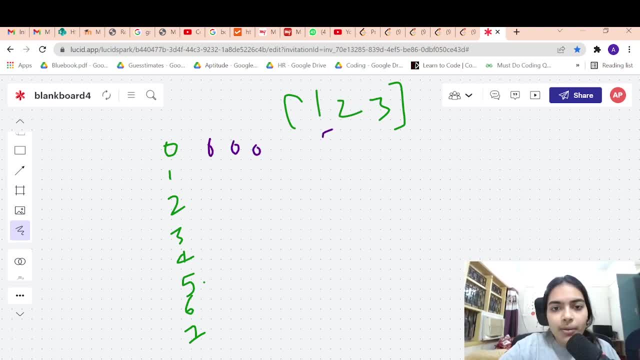 There are three elements, so 0, 0, 0.. So I get an empty subset. Now let me write the binary representation for 1.. It is very simple, right? It is simply 1, right? So it is simply 1, 0,, 0, 1, okay. 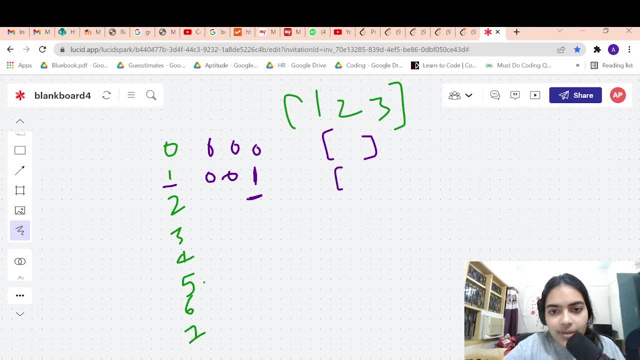 So let's say, corresponding to this, I take a number, I take the subset 1, okay, I just take the first element. okay, and so on. Let me write the binary representation for 2.. So the binary representation for 2 is 0, 1, 0. 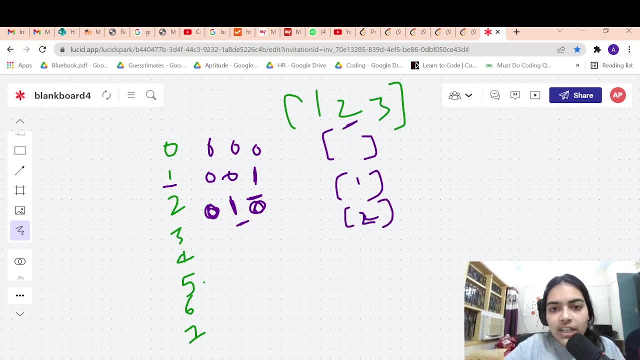 So it will give me the subset 2, okay, At this position, whatever number is there, I will take that and I will not take any other numbers. Let me write the binary representation for 3.. 3 is just 0, 1, 1, right, 3 is 0, 1, 1.. 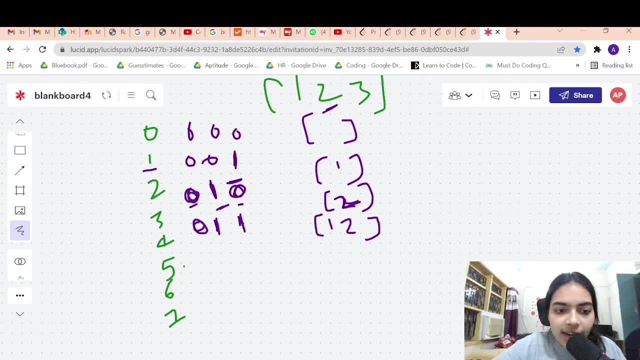 So I am going to take 1 and I am going to take 2,. okay, Let me write the next binary representation for 4.. 4 is just 1, 0, 0.. So I have the subset 3.. 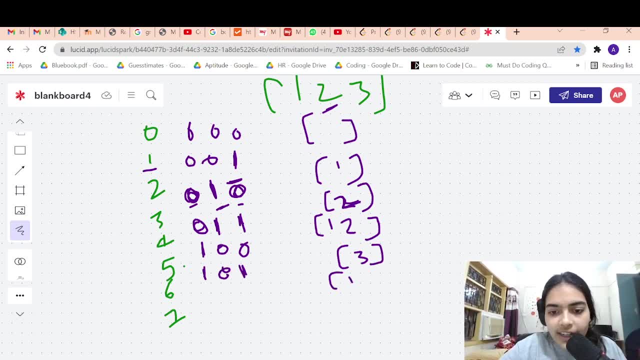 Let me write the binary representation for 5.. 1, 0, 1.. That means I take 1 and I take 3.. Let me write the binary representation for 6.. 6 is what 4 and 2.. 1, 1, 0, okay. 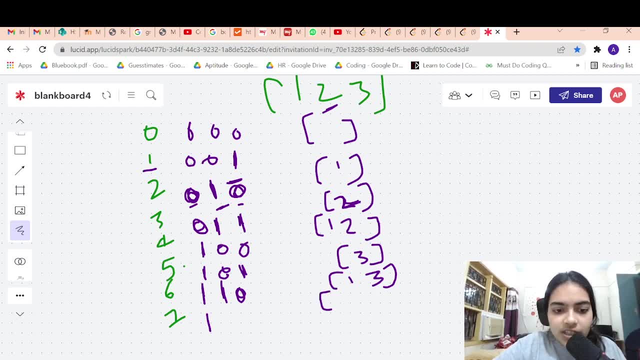 1, 1, 0 means I take 2 and I take 3.. Binary representation for 7 is 1, 1, 1.. that means i take all the numbers, so one, two, three. so we can see that we have generated all. 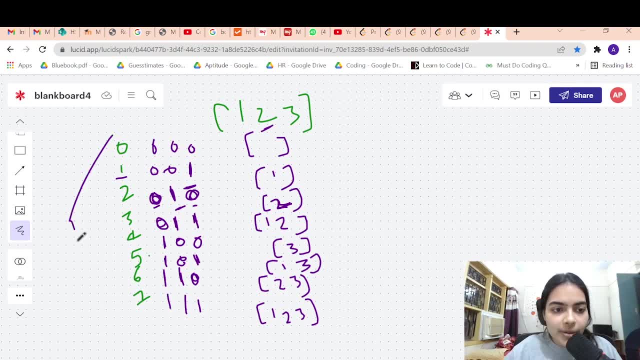 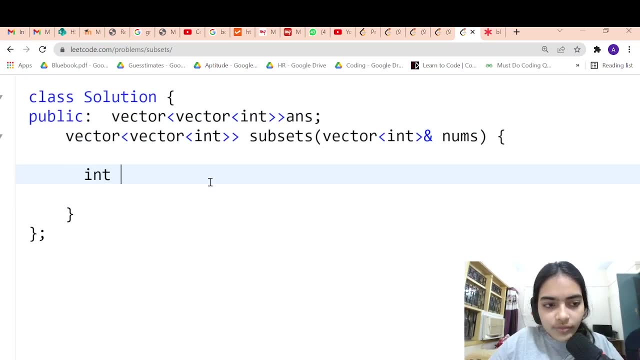 possible subsets using just binary representation of all numbers, from zero to two, power n. so that's what we are going to do. okay, so let's write the code. so what we have to do. first, let me get the size, nums, dot size, right. in our example, n is equal to three. so if n is equal to three, we will have 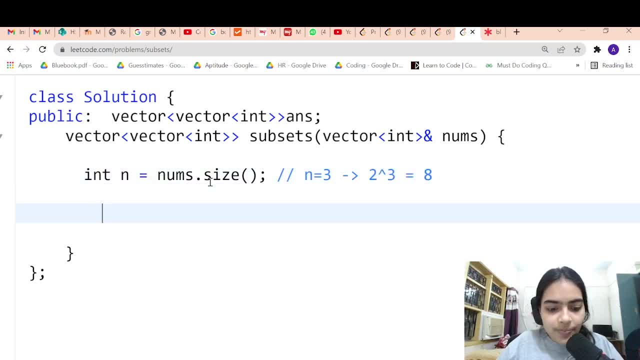 two power three subsets- right, so we will have eight subsets. okay, now let me iterate for all numbers how many subsets we have to generate. two power n- right, so i can either write: uh, two power n. like this: so if i use the power function, power function- i get two power n. right, so i can generate. 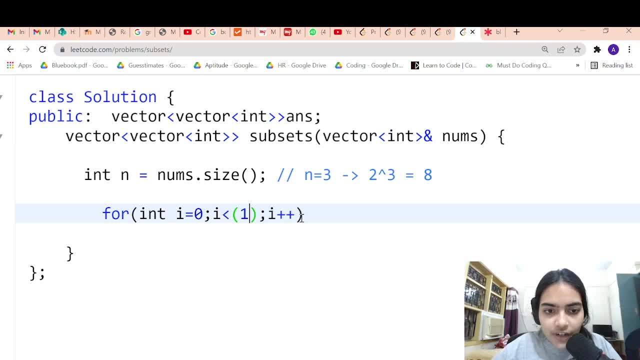 all the subsets. one more easier way of writing this is: you just left shift one n times, right? so if you left shift once, it will multiply by two. if you left shift by n times, it will multiply n times. so, uh, so, every time it's multiplying by two, so it will multiply n times. 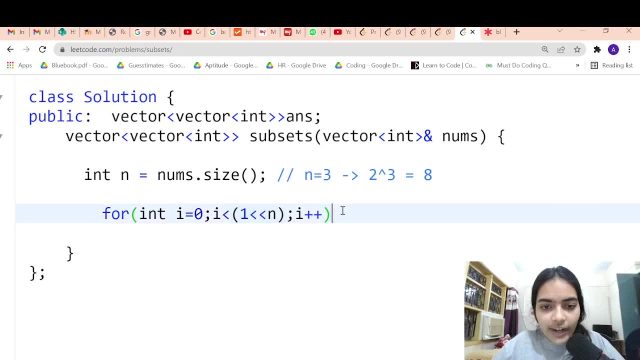 by two, so it will give two power n. so this is also same, just to write two power n, okay, in using uh left shift operator. okay, now, what we are doing, this is going to generate all the numbers, right, so what your? i will be, i will be zero, then i will be one, i will be two, i will be three, okay, so 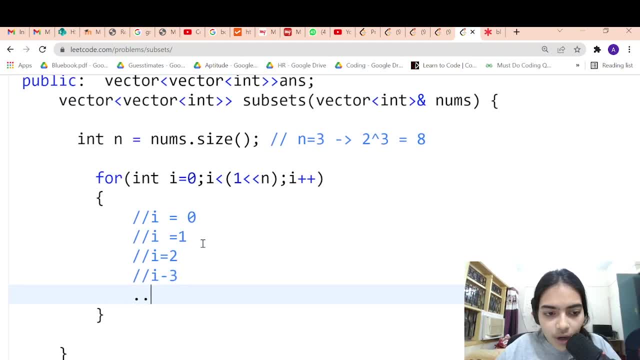 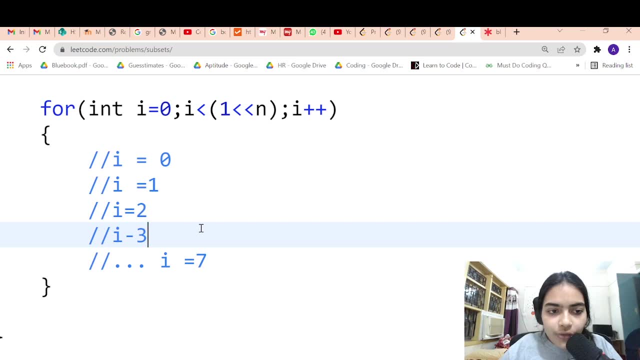 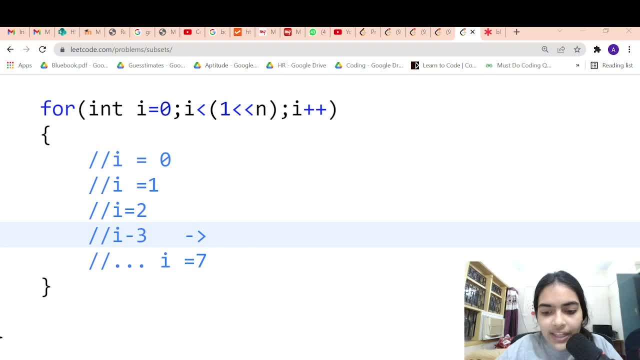 let's. let's consider the example, for i equal to 3, for example, i is equal to 3. what is the binary representation of this? i is equal to 3 means you have 2 and 1, right. so the binary representation is simply 1- 1 for that, okay. and here you have 0, so 0, 1, 1, so whenever, okay. so what does this? 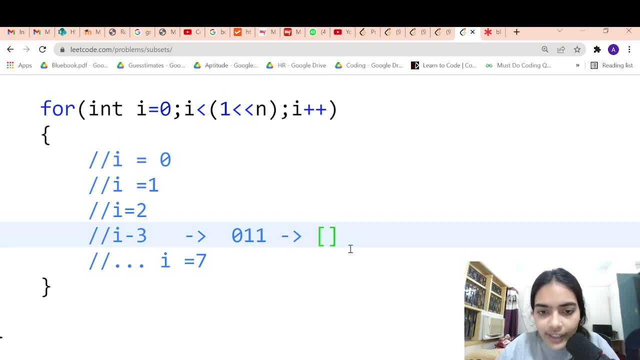 corresponds to: if you have 1, 2 and 3, right. if you have 1, 2 and 3, you are going to take the elements right. you are going to take the elements which are at the zeroth position and at the first position. that means you will take these two elements. this corresponds to the subset 1 and 2 right. 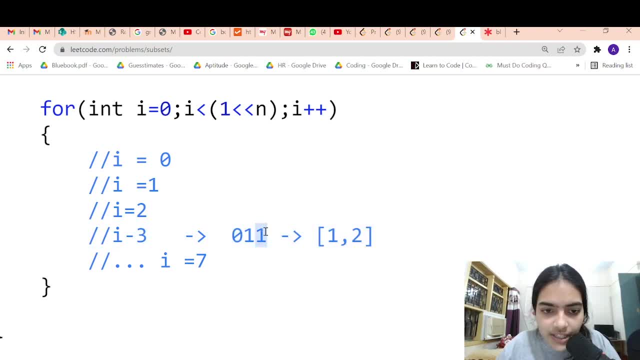 so this corresponds to the subset 1 and 2, because at the zeroth index, whatever element is there, you will take that. at the first index, whatever element is there, you will take that. at the at this index, whatever element is there, you will not take that. so this this element will be. 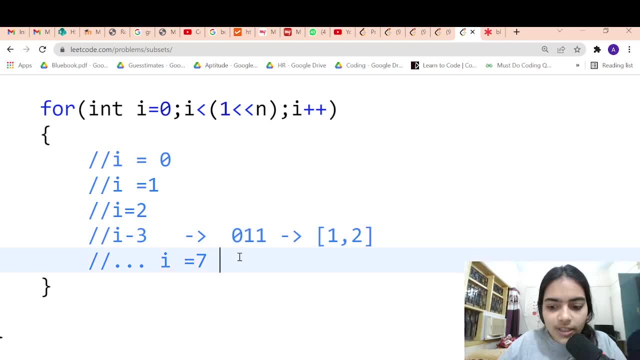 gone and you will take only two elements. this corresponds to 1- 2. similarly, for i equal to 7, this corresponds to 1, 1, 1. you are going to take all elements. so this corresponds to the subset 1, 2, 3. okay, let's see, for i equal to 2, for i equal to 2. 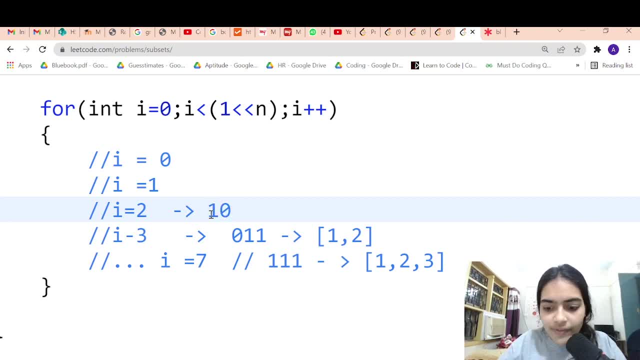 what is? the binary representation is just 1, 0, right, and you have 0 in the beginning. so this means you are going to take the element at the first index. so you are going to take the element. you have 1, 2, 3. so just take the element at the first index, which is 2. okay, so this corresponds. 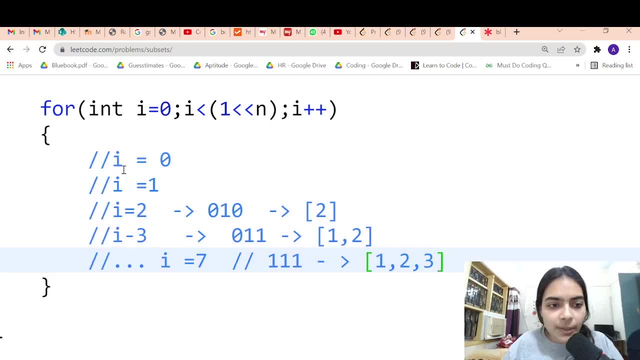 to the subset 2 and so on, so corresponding to every binary representation. right, you will be able to get a subset, so let's generate that subset now. okay, so let me erase this and let's generate the subset. so for int, j equal to 0, j less than n, j plus plus. now what we are going to do. 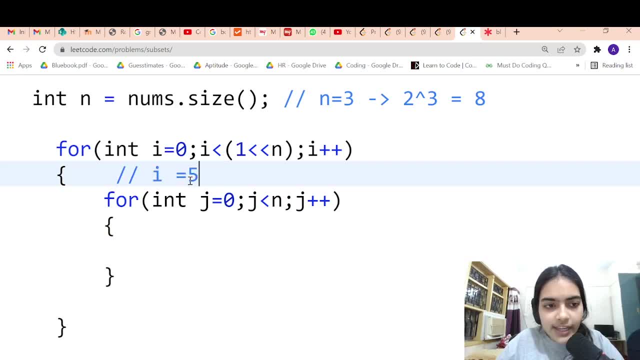 we are going to generate the subset. okay, let's take an example. okay, let's say i is equal to 5. let's take last example. so when i is equal to 5, you have 4 plus 1, 5, right? this is the binary representation: 1 0- 1. so you have to check which bit is set. if this bit is set, for example, see: 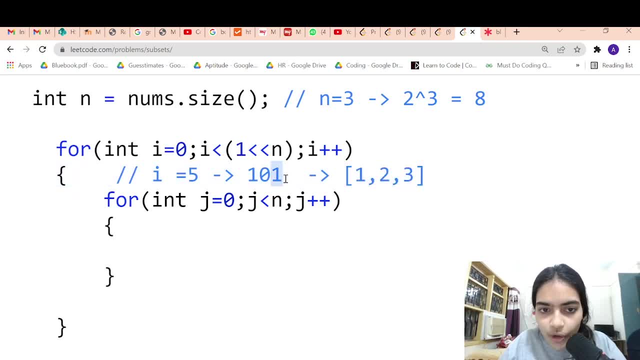 what? what does this corresponds to 0, 1, 0, 1, 0 E&k. this corresponds to: you take the number at the at the 0th index. this 0 means you don't take the middle number and you take the number which corresponds at the second index. again, okay, 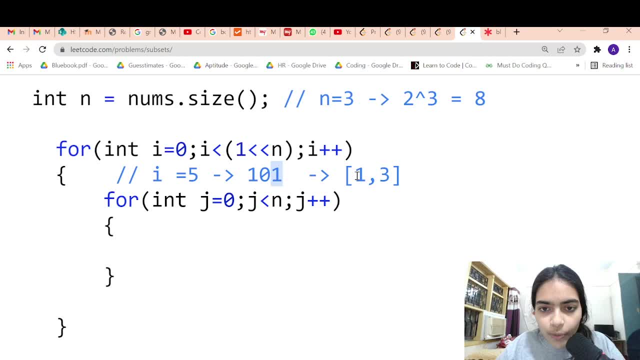 so this corresponds to the subset 1, 3. this 1 corresponds to this 1 and this 1 corresponds to this 3. okay, we are eliminating 2, we are not taking 2, because this is 0. so what we are doing is we are checking whichever bit is set. okay, so what you have to do? so, if see, you have to check. 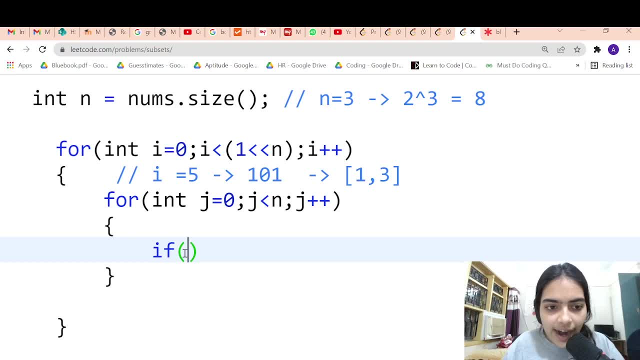 whether the bit is set. so how will you check if the bit is set? just take a and right. so let's say we left shift 1 j times, right. so first what you will do: you left shift 1, 0 times. so you are going to check the, whether this bit is set or not. last bit is set, okay, and you take the and of that with. 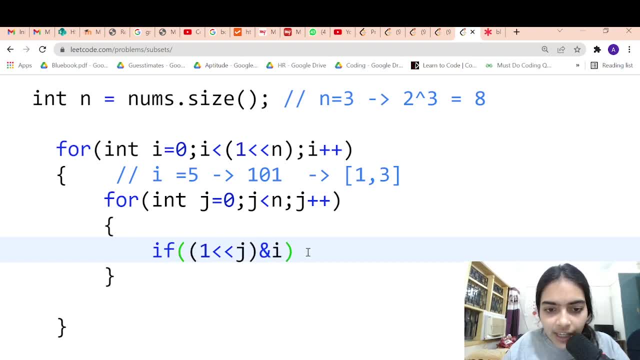 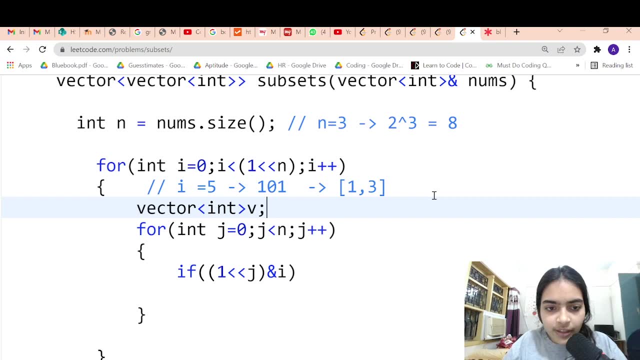 i. so if you take the and of that with i, if this bit is set right, then you can take that element. so let me take a vector, vector, int, v, and, and, and. if this bit is set, so you are going to push that, push in terms of j, right, and then you can. 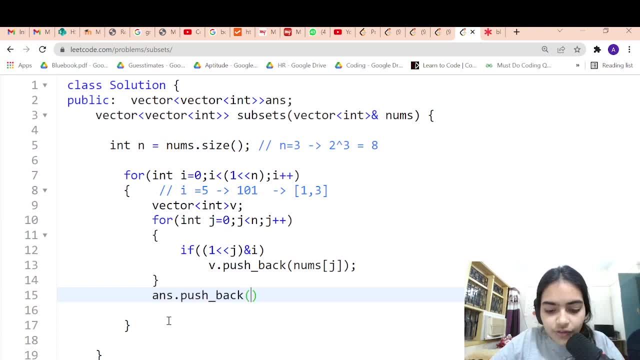 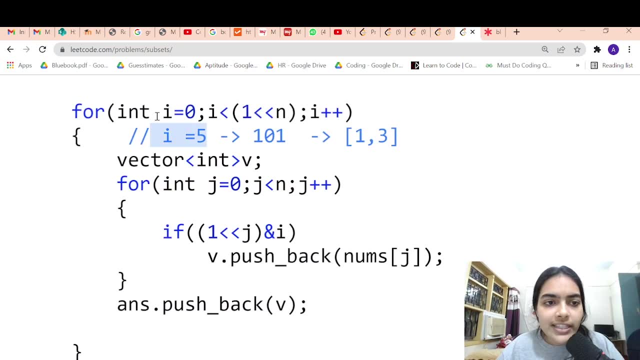 push it in answer. so then answer dot, push back v and finally you can return. answer. that's it. this is a simple code. okay, let's let's discuss it once more. see when let's say: let's take an example, so i will range from 0 to 7. okay, let's take the example, for i equal to 5, the binary representation. 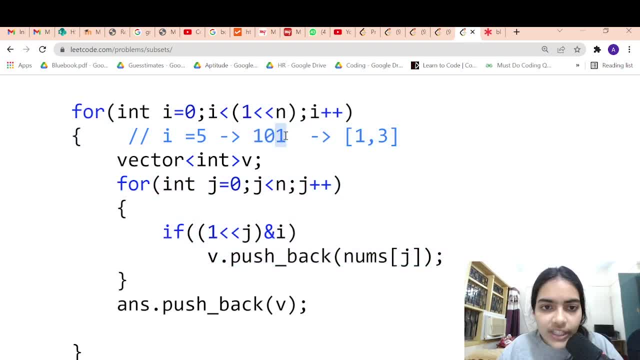 is 1, 0, 1. so what we are doing in this for loop corresponding to this one right. so this is the binary- represents corresponding to this one right. so this bit is set in i. this is the. this is i right. so in i the zeroth bit is set right. so when 1, you are left shifting 0 times, you just have the, you just. 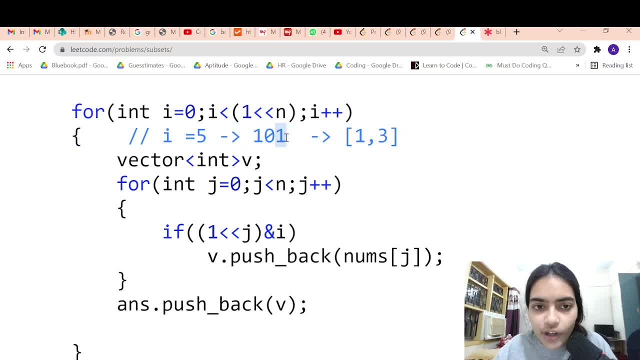 have this. you just have the first one. you are checking if it's set or not. so it is set. right, this is set. so in this case, you are going to push in nums, you are going to push the first element, so you will push 1. okay, next time. next time this was for the case- j, equal to 0. next time, j is equal to. 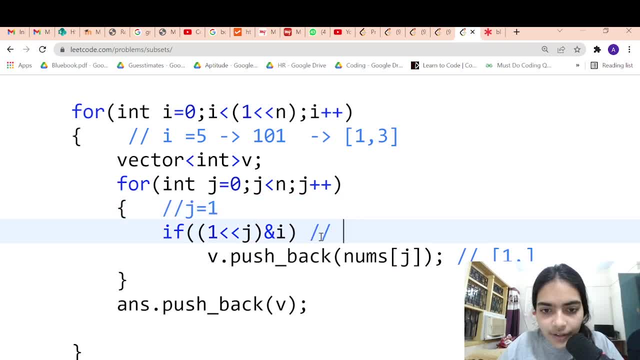 1. so what you will do, you will left shift 1, 1 time, right, so this will just left shift 1 with 1 time. so you are going to do, and of okay, so 1 left shift 1 times will give you 1, 0. and what is i? i is equal to 1, 0, 1, so you are going. 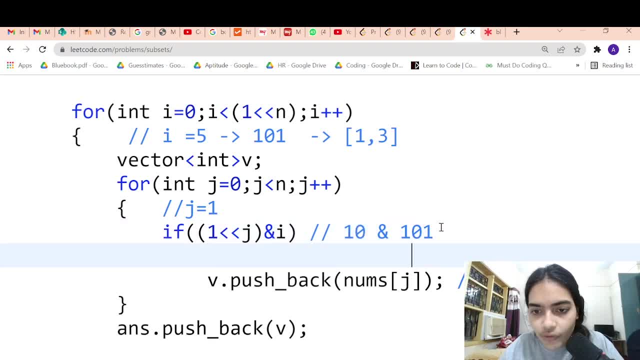 to take and of 1: 0 and 1 0, 1. see if i take and of 1: 0 and 1 0, 1 and and with uh and with 1: 0, what i am going to get. if i take the and of these numbers, i am going to get 0 because because 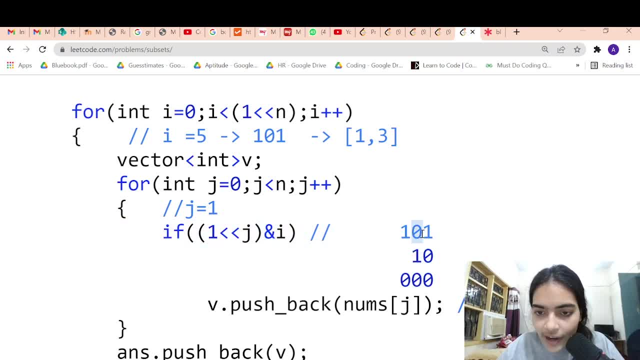 this bit is not set right. this bit is not set, so, and of 1 and 0 will give me 0 only. anyway, everything else will be 0, right? so this bit is not set, so this will be 0. so that's why i will. 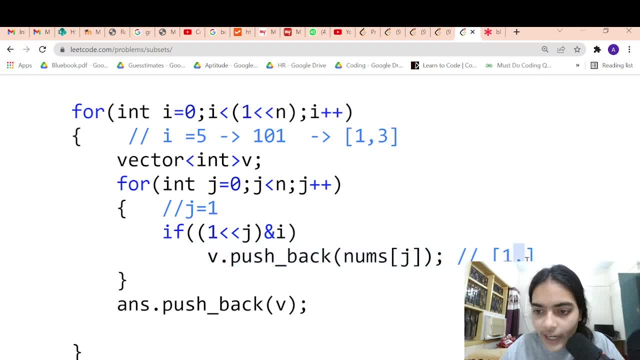 not push. i will not push the second element. the second element will not get pushed. okay, next, next time. j is equal to 2, right, so what i will do? i will left shift 1 2 times. so what will i get? i will get this number 1 0, 0. see, this is 1, right. i am left shifting by 2 times, so i 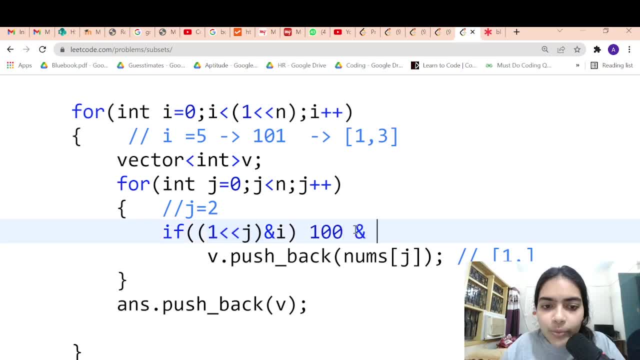 get 1 0 0 0 0. this corresponds to 1 left shifted by j, and i am going to do and with i. what is i in our example? i is 1 0 1, right, i is equal to 1 0 1, so i am going to take and of 1 0 0 and 1 0 1, so basically i am. 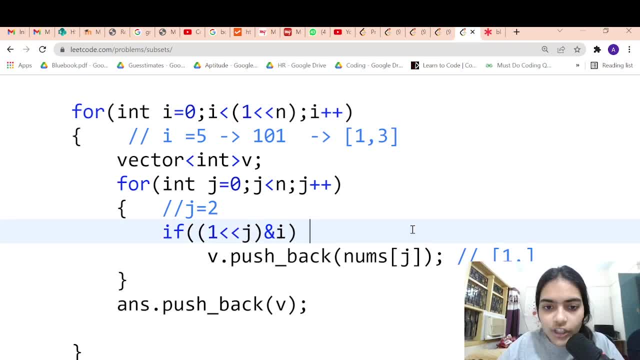 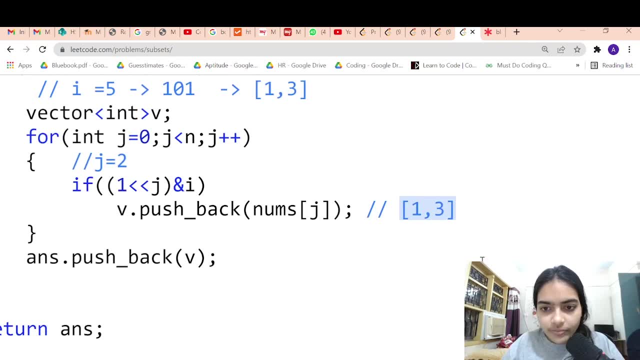 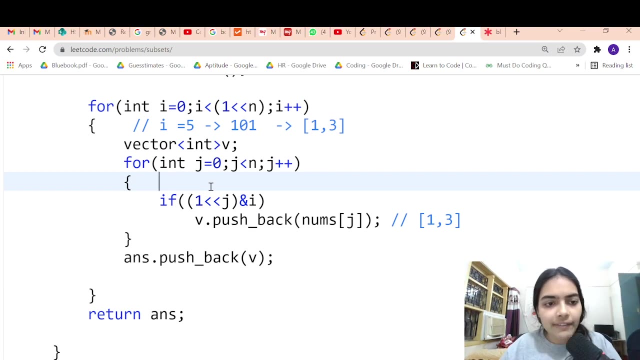 just checking whether this bit is set or not. so this bit is set right. it will be a non-zero number. that's why i will push the number at the index of at this index. so i will push 1, 3, so so i will have 1- 3. next time j will be equal to, next time j will be equal to 4, and so on. right, i will keep. 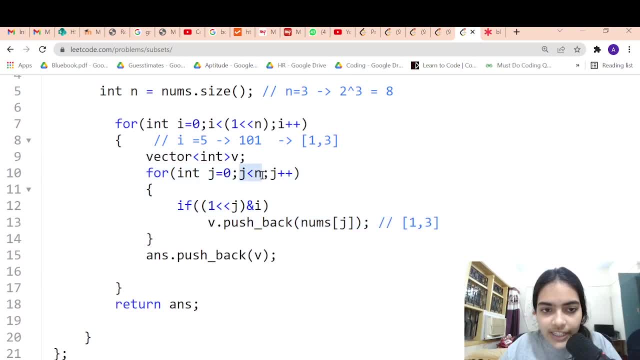 doing this, j will not be equal to 4, because when j is equal to 4 it will exit the loop right. so i have to just check: j is equal to 0, j is equal to 1, j is equal to 2 and that's it. when j becomes.